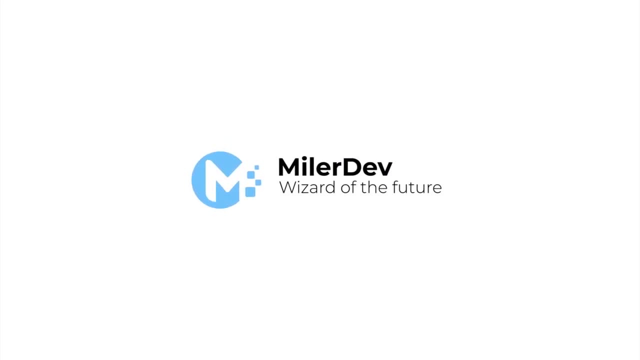 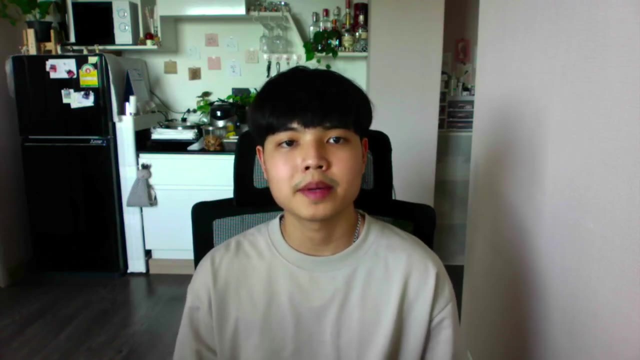 What's going on, guys? Welcome to my Ledev channel. In this video, we're going to learn about the difference between event handlers and event listeners in JavaScript. In JavaScript, an event can be a button click or a mouse hover over. It is important to respond to the event by showing a. 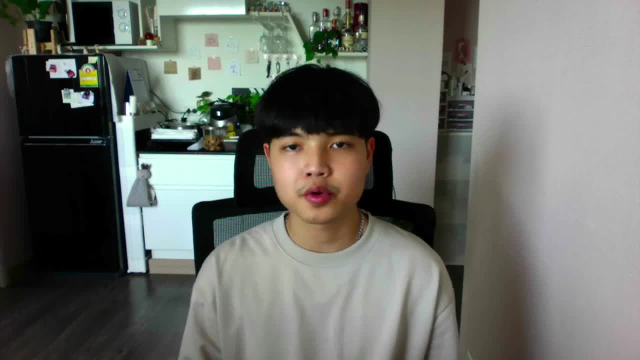 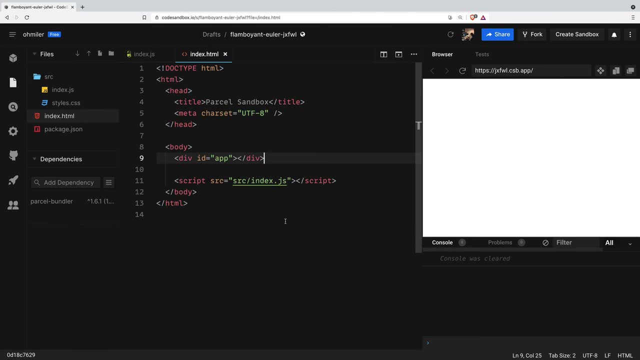 model when a button is clicked. Today you will learn the two ways to handle events in JavaScript in a nutshell. In JavaScript, you can handle events in one of two possible ways. First, we can use event handlers. Second, we can use event listeners. So to use an event handler, we can use: 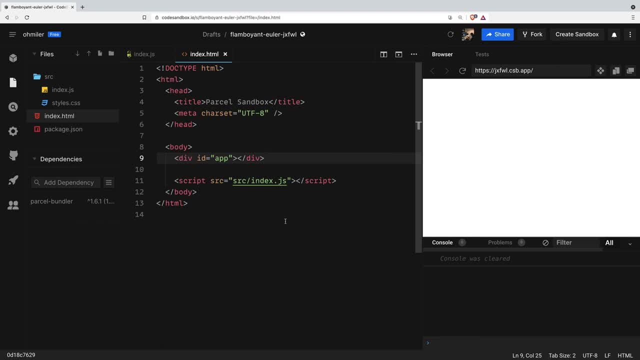 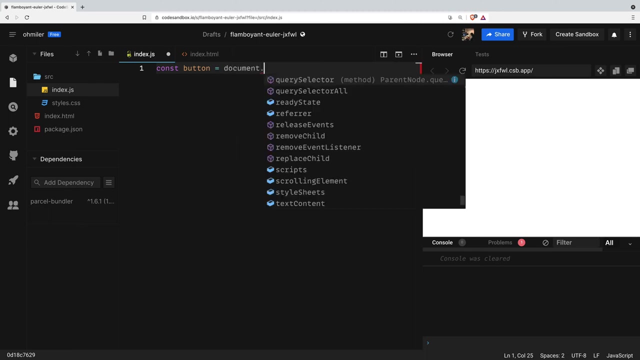 one of the event handler properties of an object. Alright, let's look at the example of using onClick event. First of all, we need to create a button and then class btnButton and next switch to the indexjs file. So we're going to create a button variable and use documentquerySelector to get the 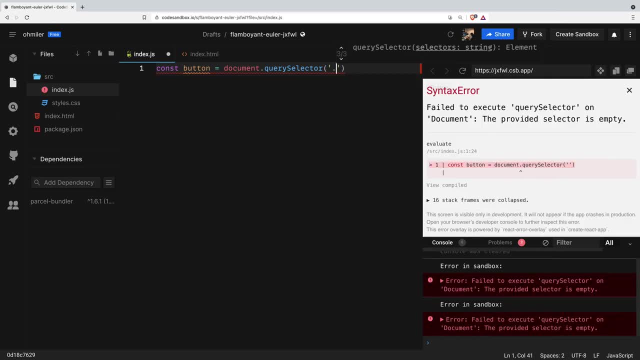 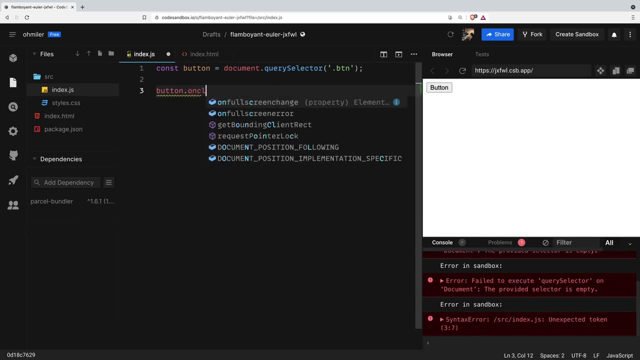 class of the button. So we're going to get classbtn, Okay. next we're going to use the button variable and then we're going to use the onClick event handler and we're going to return consolelog button clicked. Alright, hit save. 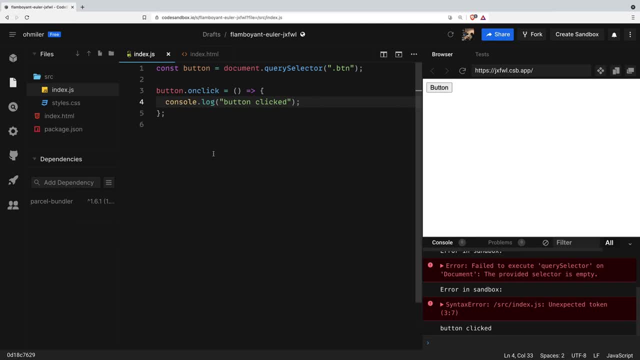 Next let's click the button. So right here the onClick event handler is triggered when a user clicks on a button. As a result, button clicked right there hits output into the console. So in the next example we're going to use event listeners. The other option to handling events is: 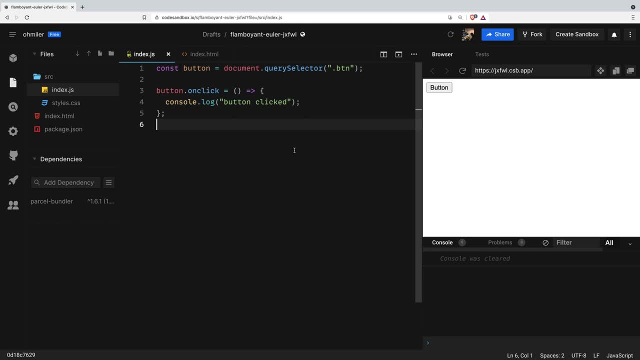 by using event listeners. An event listener is something you assign to an object. As the name suggests, the event listener listens for events and gets triggered when an event occurs. Okay, let's repeat the previous example by assigning an event listener to a button to listen for clicks. 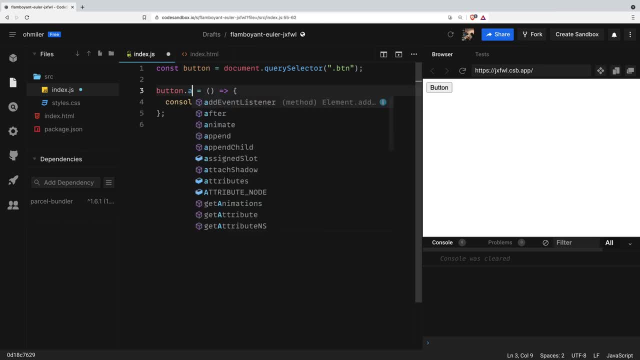 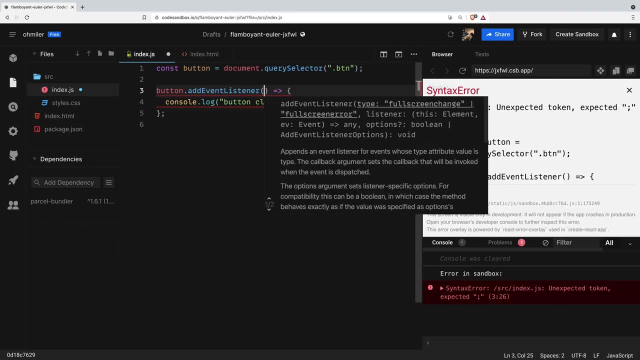 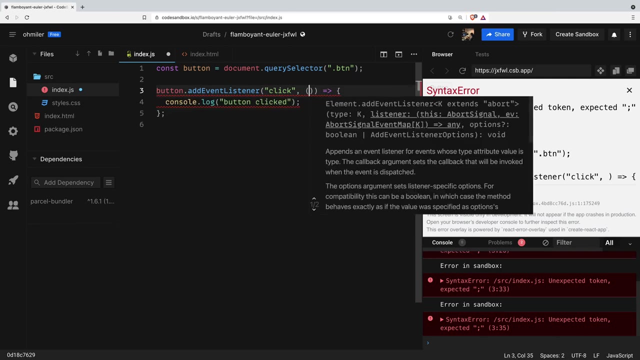 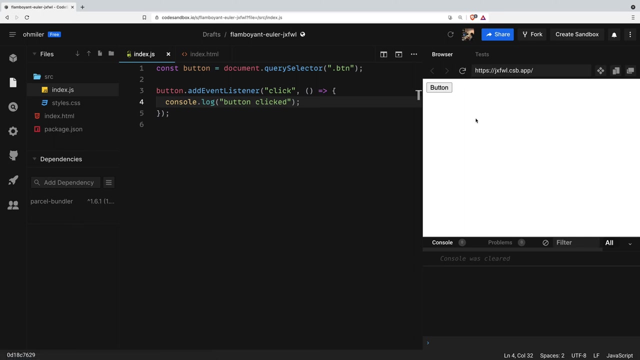 Alright, we're going to change onClicked to addEventListener and then we're going to change our code here for listen to click event and return Alright and refresh the page. So let's click on the button Now. clicking the button triggers a click event, which in turn runs. 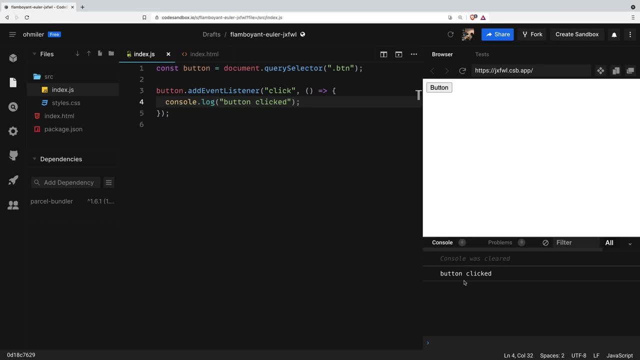 a block of code which outputs button clicked to the console. right there, The minor difference between event handlers and event listeners is easy to understand. You can only have one event handler for a specific event type, but you can add multiple event listeners for it. Okay, let's see. 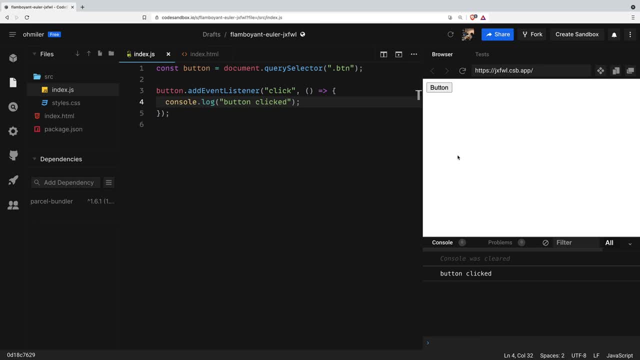 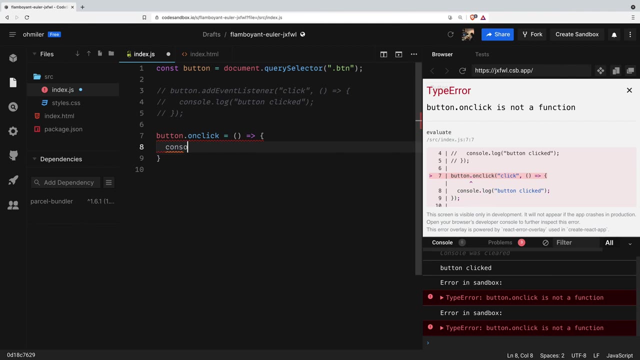 what happens if you try to add two onClick event handlers to the same object. So let's click on the object. we're going to comment this code and then copy. So I'm going to change this to: onClick return consolelog: first event handler. 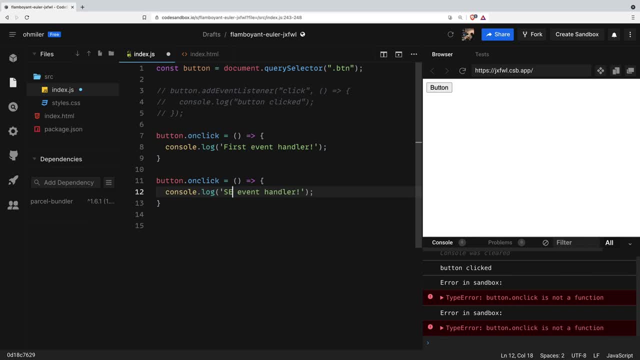 and copy. this is second event handler. Alright, hit save And then you click the button. So right, object can only have one event handler for each event type. the first on click handler gets over written by the second. this results as you can see in the console here. all right, let's repeat this. 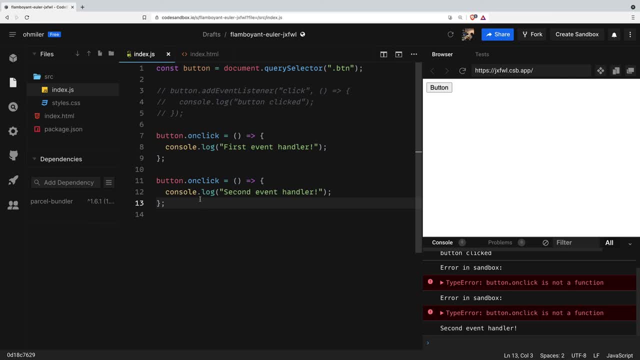 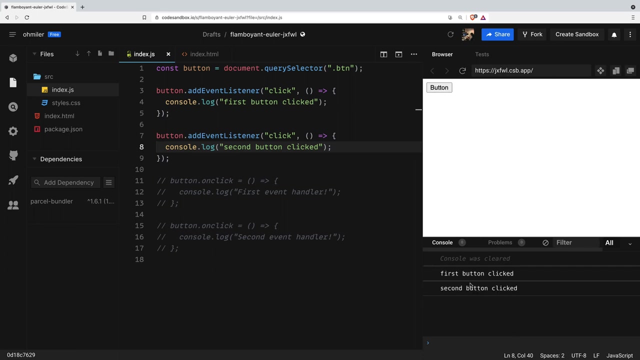 experiment by using two click event listeners. we're gonna comment this code and uncomment this, so copy and we're gonna change to: uh, first button click and second button clicked and then refresh the page and hit the button. as you can see in the console, it is okay to have multiple event. 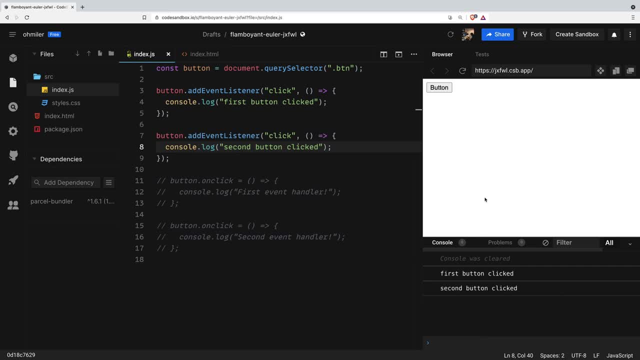 listeners of the same event per object. thus both of the listeners are triggered once a button is clicked. i believe right now a lot of you guys have wondered which should i use. generally, it is advised to use event listeners over event handlers, because you can add multiple event listeners for. 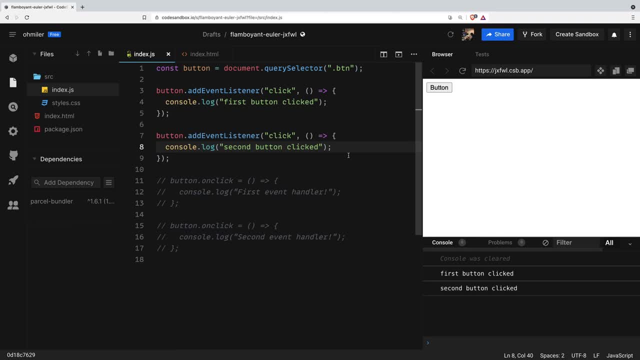 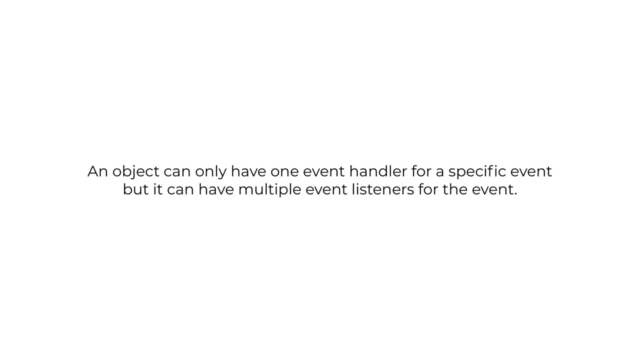 the same event. conclusion: event listeners and event handlers are used to handle events such as button clicks on your page. there's a subtle difference between event listeners and event handlers. an object can only have one event handler for a specific event, but it can have multiple event listeners for the event. when in doubt, prefer event listeners over. 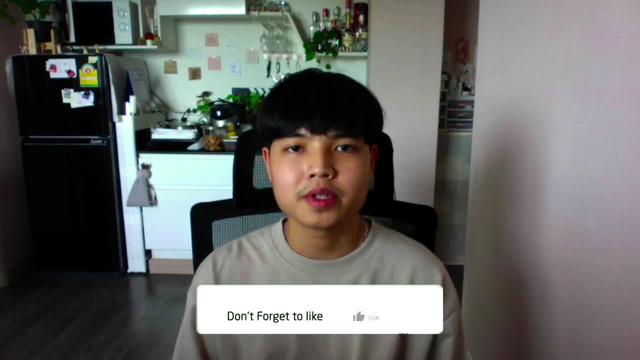 event handlers. alright, guys, that's it about this video. i hope this video is helpful to you guys. if this video is helpful, don't forget to like and subscribe, and see you guys soon in the next video.